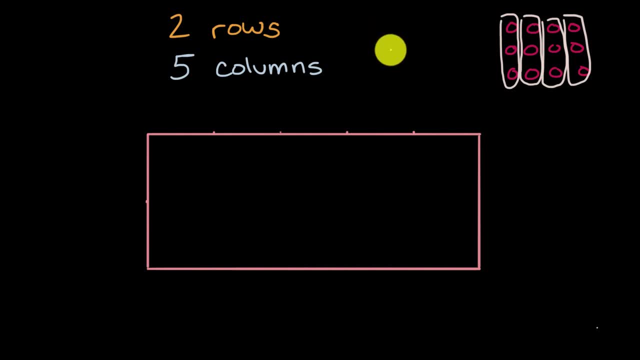 So, now that we understand what rows and columns are, let's first think about, maybe pause this video and think about how would you divide this rectangle into two rows? Well, the way that I would tackle it is I would draw a line that goes from left to right. 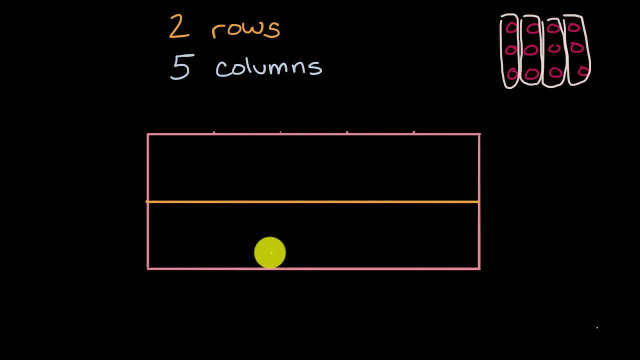 And there you have it. I now have the rectangle split into one row and now a second row. Now pause the video and you could draw this if you have a pencil and paper with you, or you could just think about what I should do. 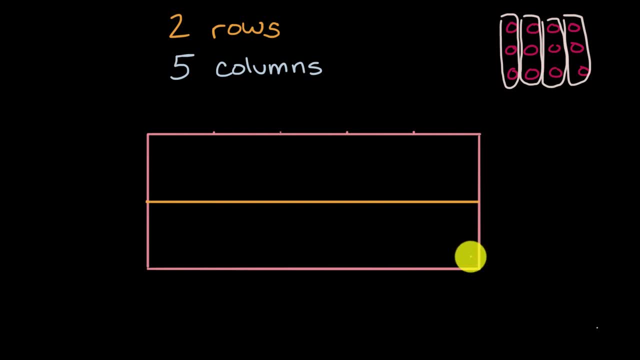 How would I now divide this rectangle into five columns? Well, what I could do is make a bunch of lines that go from top to bottom. So that's one column there. This is a second column, This is a third column, This is a fourth column and a fifth column. 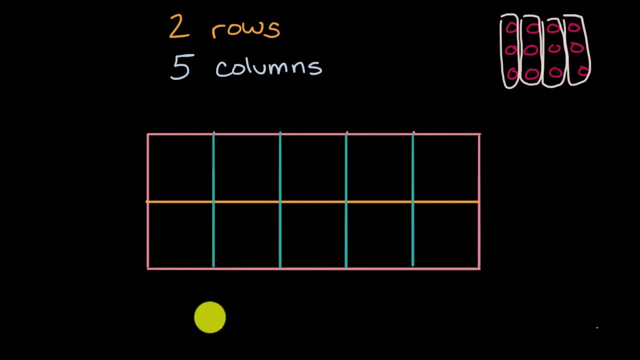 So there you have it. I have two rows, one row, two rows, and I have five columns: One, two, three, four, five. Now what's interesting is when I split the rectangle in this way into two rows and five columns.